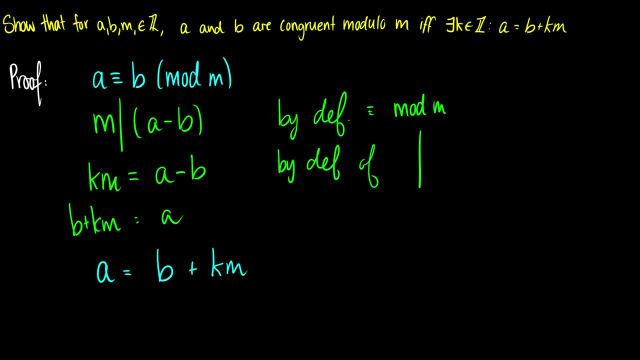 and plus the others to find them out. So let's get an example, that one task and get another one, but a is equal to b, So we're going to get b plus km is equal to a and that's exactly equivalent to our last line. So if you go down, then that is the left to right direction. If you work up, 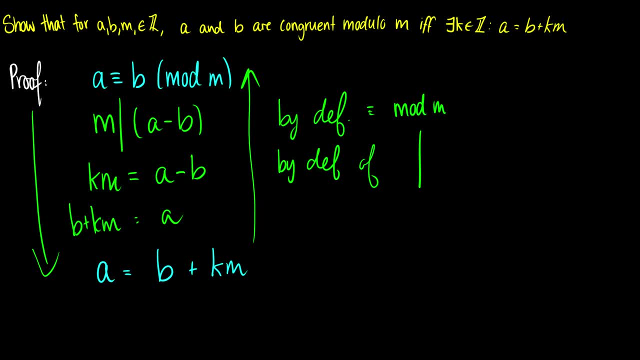 that is the right to left direction. So that is the proof that if they're congruent, modulo m, then you can write one in terms of b plus km. Okay, so this makes sense, because we're saying this integer a times. it goes in properly, so that's b. 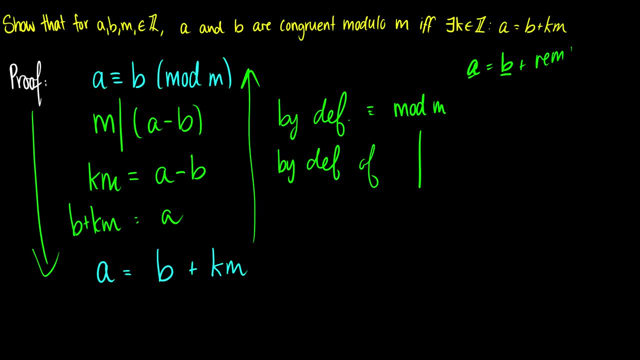 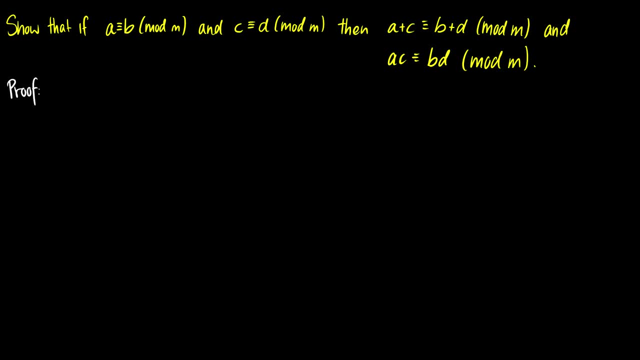 plus k times m. so this is kind of like the remainder. Okay. so, with that being said, let's prove something more. So if a is congruent to b mod m and c is congruent to d mod m, then a plus c will be congruent to b plus d mod m. 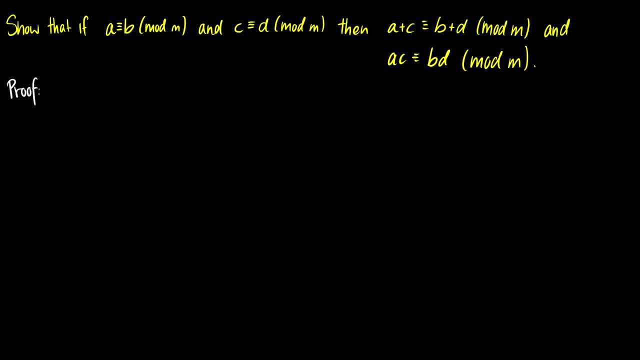 and a times c will be congruent to b times d mod m. So let's prove the first one here. So we have a is congruent to b mod m. so we know we can write this as: a is equal to b plus km. 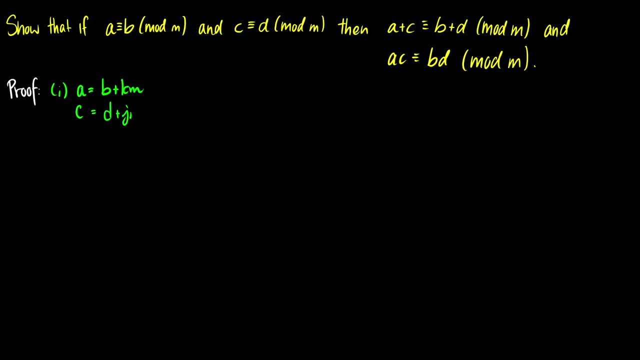 and we can write c equal to d plus jm. So last time we proved that we can do this, They are congruent to each other, so we can write them in terms of b plus k times m. Okay, so we wanna show that a plus c. 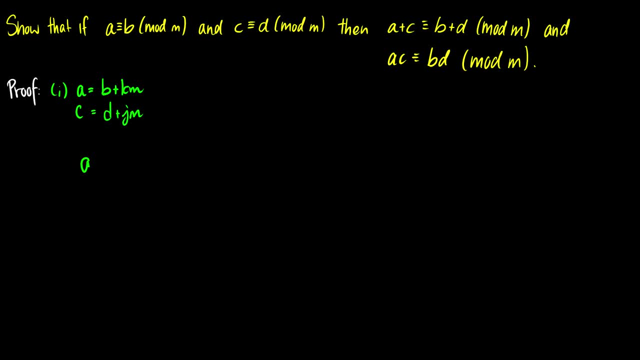 is equal to b plus d mod m. Okay, so a plus c is the same thing as b plus km plus d plus jm. So let's move together like terms. So let's move b plus d together, and then km and jm. let's put those together. 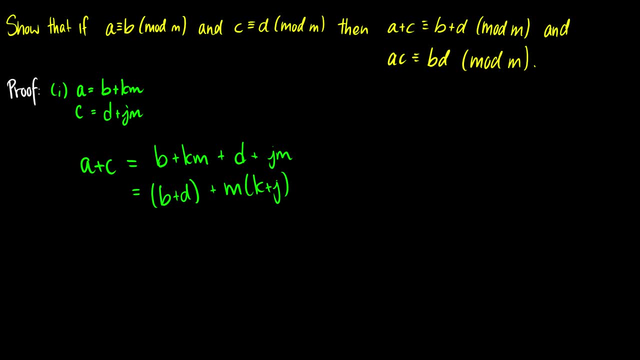 So if we do that, we can factor out a- k. So now we have that a plus c is equal to b plus d plus m times k plus j. Well, because of our proof earlier, this implies that a plus c is congruent. 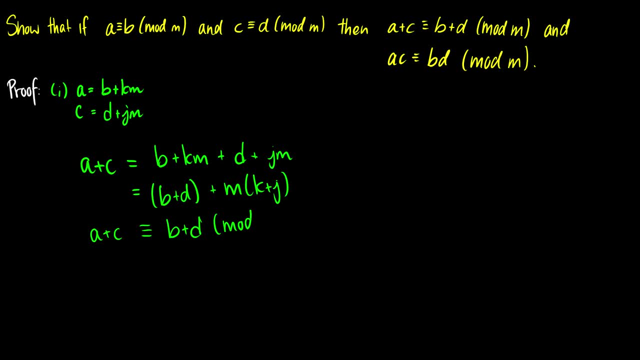 to b plus d mod m, And it's the same formula. So before we had, a is equal to b plus km. Well, here's our a. our a is a plus c, our b is b plus d and our k is our k plus j.